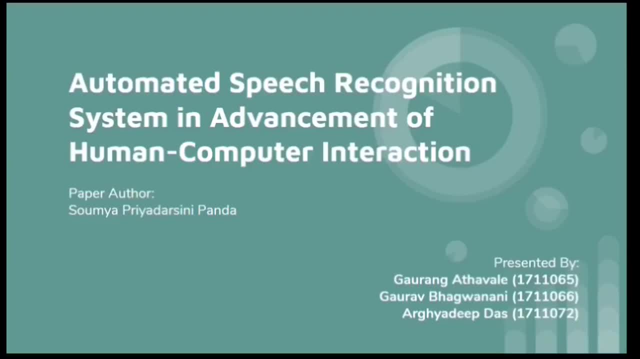 Hello everyone. Today I, Argyadeep Dutt, along with my friends Gaurav Nathavale and Gaurav Bhagwanani, will be talking about the research paper Automated Speech Intermission System in Advancement of Human-Computer Interaction. 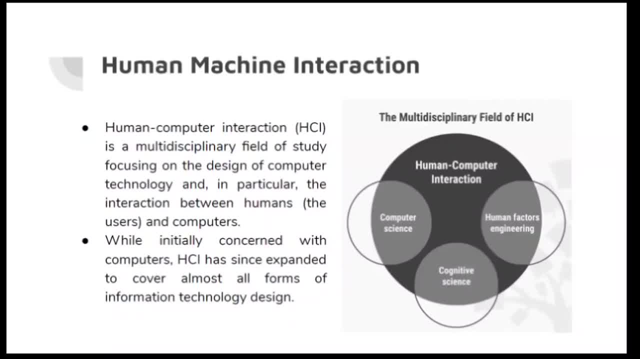 by Soumya Priyadarshani Panda. So let us first understand about what exactly is human-machine interaction or human-computer interaction. So human-computer interaction is a multidisciplinary field of study that focuses on the design of computer technology. 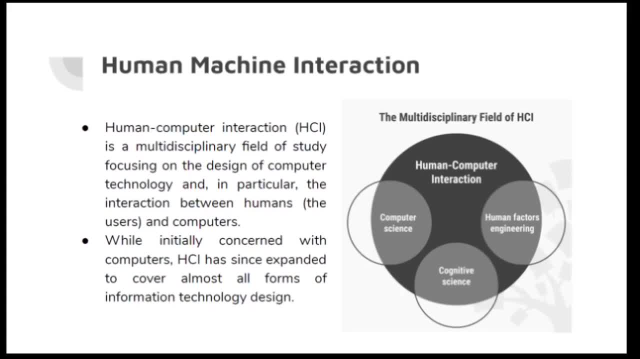 and specifically the interaction between the humans and the computers. So, as you can see the diagram here, we can see the interaction between human-computer interaction field with computer science, human factors, engineering and cognitive science. So while it was initially concerned with computers, HCI today has then expanded. 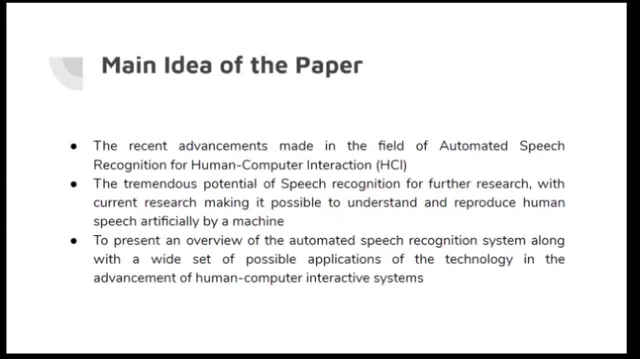 to cover all the fields of computer science and cognitive science. So, talking about the main idea of the paper, it talks about the recent advancements that have been made in the field of automated speech recognition for human-computer interactions. It also talks about the tremendous potential that speech recognition has for further research. 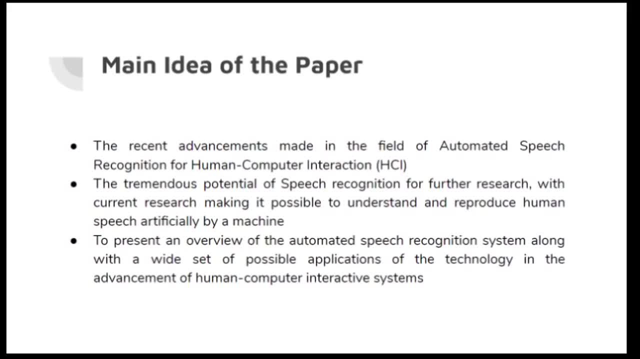 with the current research making it possible to understand and reproduce human speech artificially by a machine. The paper also presents an overview of the automated speech recognition system, along with a wide range of possible applications of the technology in the advancement of human-computer interactive systems. 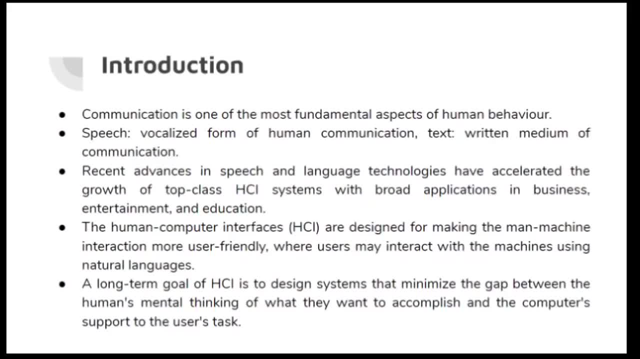 So, coming to the introduction of the paper, we all know that communication is one of the most fundamental aspects of human behavior. It can be initiated in two ways, that is, through speech, which is the vocalized form, or text, which is the written form. 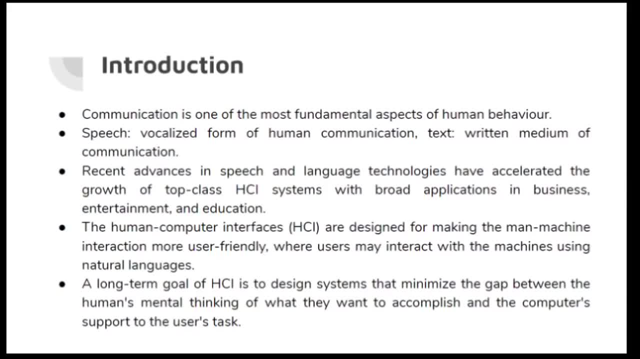 The recent advances made in the field of speech and language technologies have accelerated the growth of top-class experiences in the HCI system with broad applications in business, entertainment, health care, education, etc. The human-computer interfaces are designed for making the man-machine interactions more user-friendly. 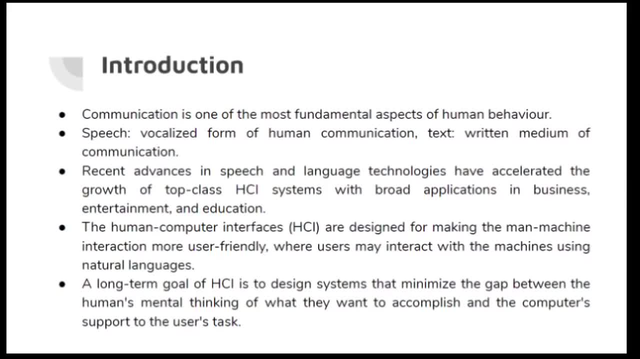 where the users may interact with the machines using natural language, for example Hindi, English, Bengali, Marathi, etc. A long-term goal of HCI is to design systems that minimize the gap between the human's mental thinking of what they want to accomplish and the computer's support for the user's tasks. 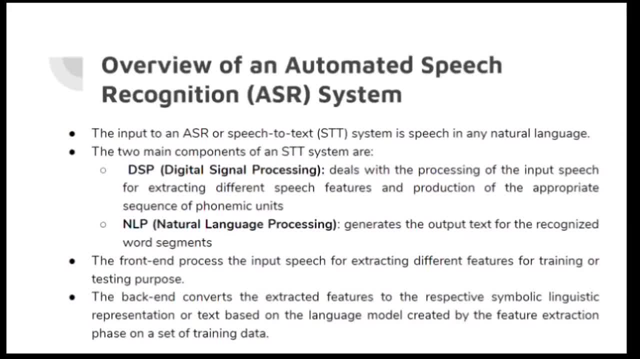 To provide an overview of the automated speech recognition system. the input to an ASR or speech-to-text system is speech in any natural language. The two main components of such a system are DSP, that is, the digital signal processing, which deals with the processing of the input speech for extracting different speech features and production of the appropriate sequence of phonemic units. 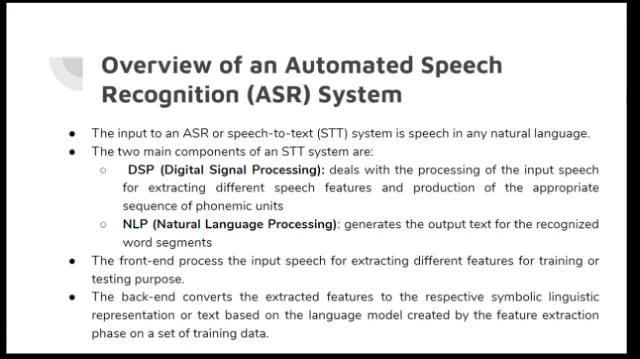 and the second part is the NLP, or natural language processing, which will generate the output text for the recognized word segments. so the system has mainly two parts, that is, the front end and the back end. the front end will process the input speech for extracting different features for 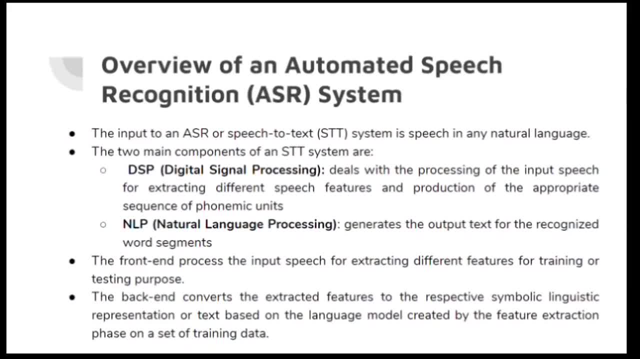 training or testing purpose, whereas the back end will convert the extracted features to the respective symbolic linguistic representation or the text or the language model created by the feature extraction phase on a set of training data. so now my friend Gaurang Athavale will talk about 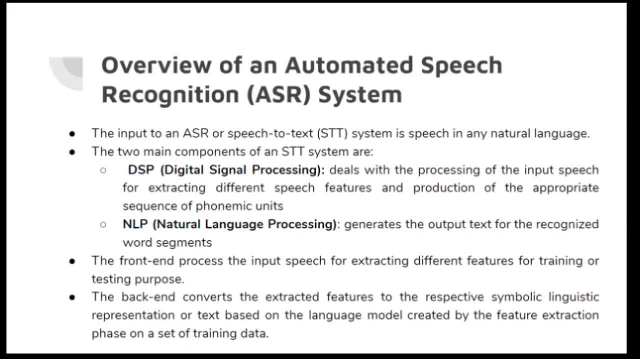 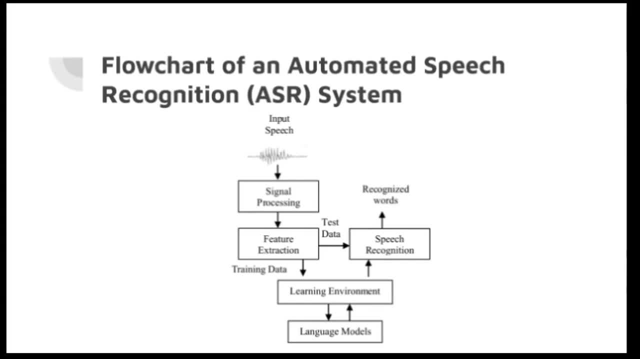 the flow of a ASR system and it's working. hello, I'm Gaurang Athavale and I will be continuing with the flowchart for ASR system. so the input speech is recorded by our application and then the signal is processed in the signal processing module. 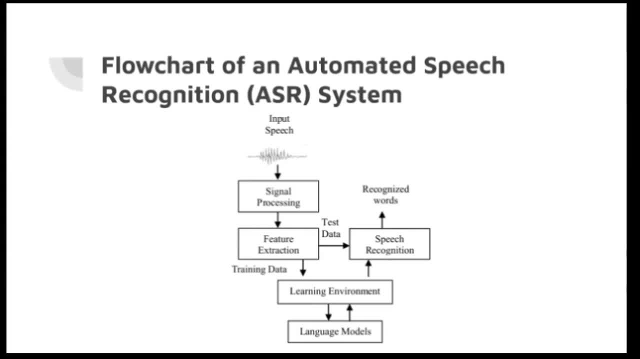 so this processed signal is further processed to extract the needed features, and then the signal is processed in the signal processing module. so this process signal is further processed to extract the needed features and it is split into two sets, that is, one for testing and one for training in training section. 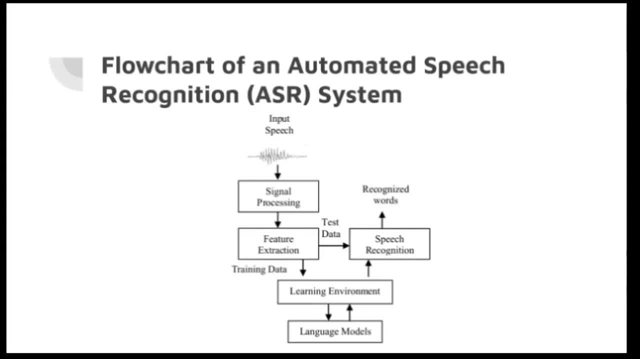 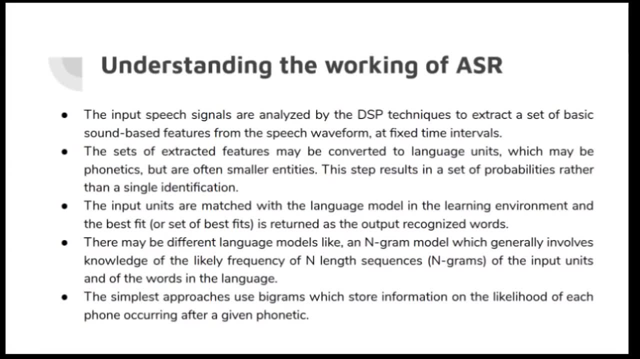 the data is trained with respect to the learning environment and finally, once the model is ready, the testing is done with the testing data set. now let's understand how ASR works. the input speech signals recorded by the application are analyzed by digital signal processing techniques for extraction of basic sound based data. 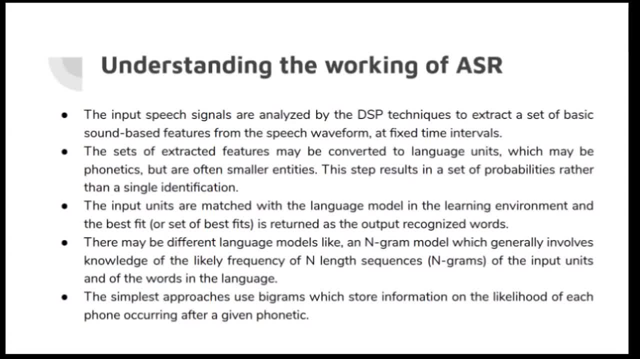 With � Tudoча respecto to sound based features, the extracted features may be converted to language units which may be phonetic. The outputs are matched with the training language model in learning environment and set of best fits are returned as the output recognized words. There may be different language models for example an n-gram model which 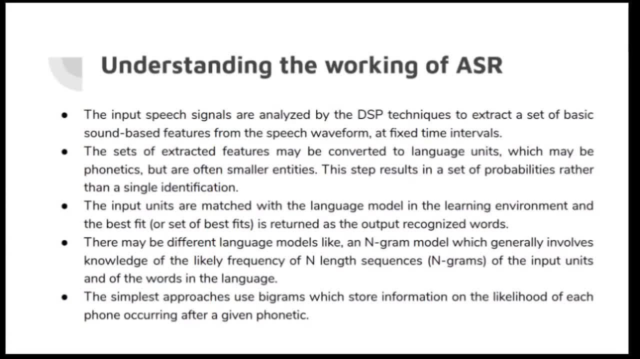 generally involves knowledge of the, of the likely frequency of n length sequences of the input units to provide a better recognition of the american language and language of the to prevent the origin All output phosphorescence and microtransmission With the input. also allows to determine National deja vu. 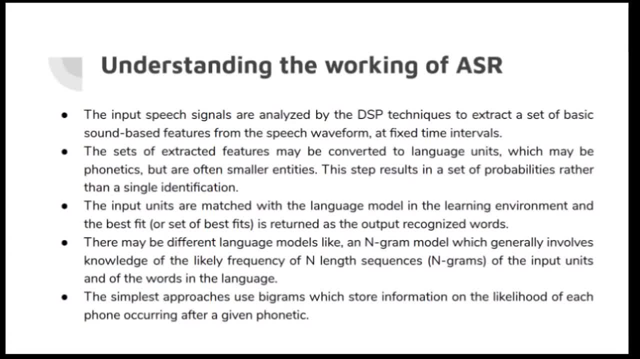 rTS and other all- spelled electure procedures to measure theälthuan length length sequences of the input units and of the words and of the words in the language. The simplest approach uses biograms which store information on the likelihood of each phone occurring after a given phonetic. 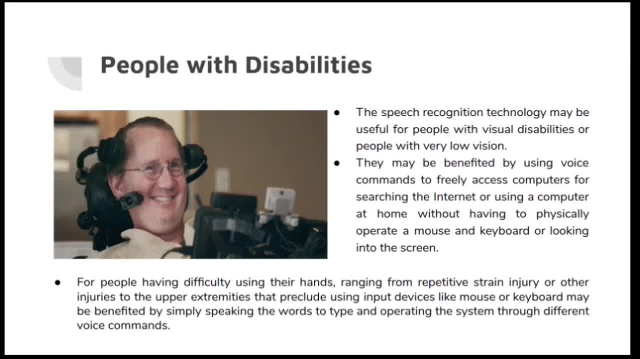 Now let's have a look at areas of application. People with disabilities: The speech recognition technology may be useful for people with visual disabilities or people with very low vision. These people may be benefited by using voice commands to freely access computers for searching the internet or using a computer at home. 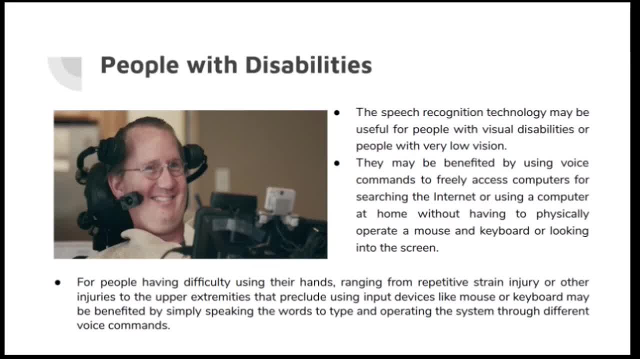 without actually looking into the screen. This will be of great use for people having difficulty using the hands or cannot operate devices like mouse or keyboard with the hands, And they may be benefited by simply speaking the words into the application over the voice commands. Now let's move on to the next application. 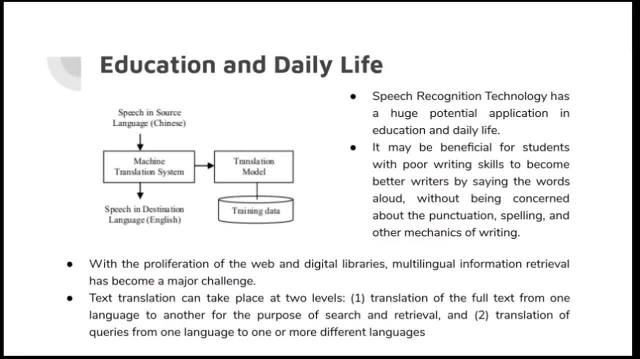 that is, education and daily life. Speech recognition technology has a huge potential application for people with disabilities. It may be beneficial for students with poor writing skills to become better writers and for students struggling with the pronunciations With the proliferation of web and digital libraries. 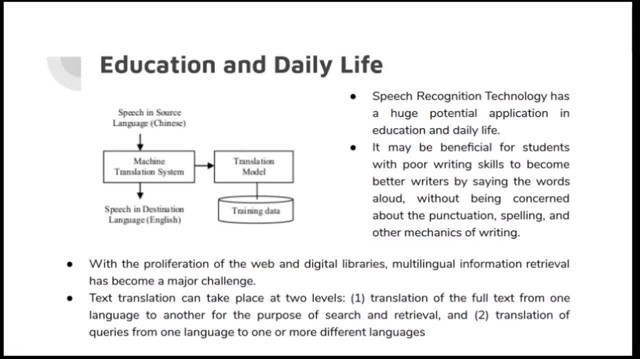 multilingual information retrieval has become a major challenge. This can be used for text translation and it can take place at two levels. First, one translation of the full text from one language to another language for the purpose of search and retrieval. And second, translation of queries from one language. 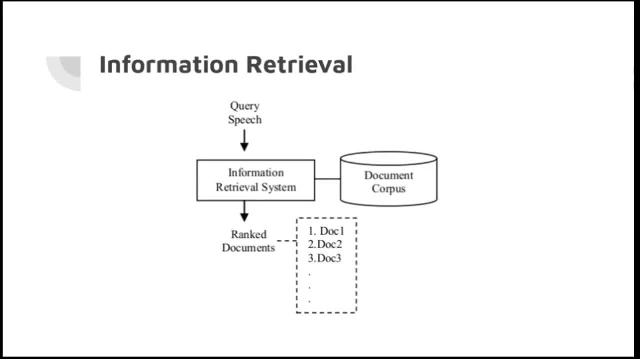 to more than one language, more different languages. Now let's have a look at information retrieval. As we can see in the diagram, that query speech is the input for information retrieval system and the output it gives is ranked documents. So in a ranked retrieval context, 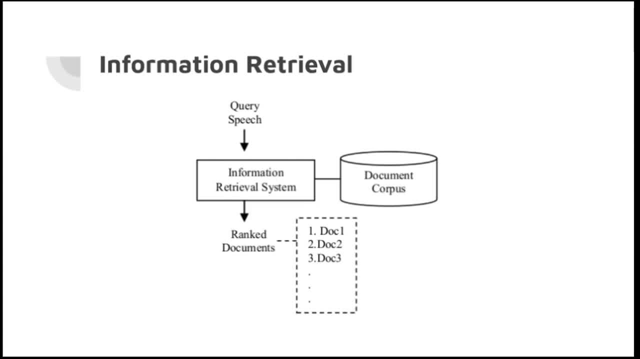 appropriate sets of retrieved documents are naturally given by the top K: retrieved documents. So if we search anything on the internet, we get some search results and these are sorted with respect to the relevance. So if we search, for example, KJSE, 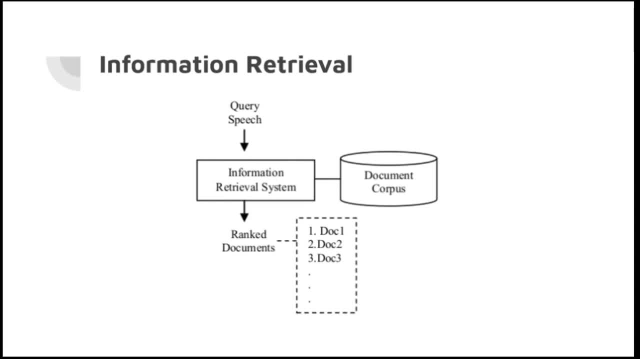 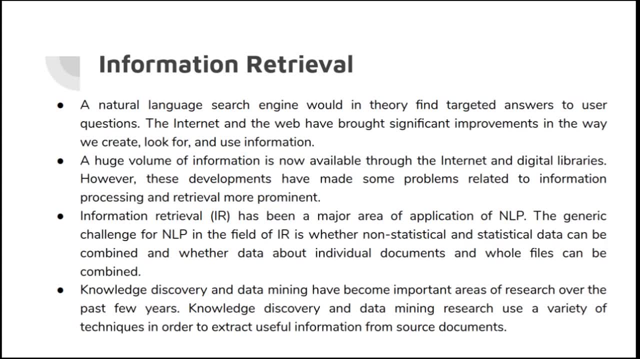 we will get our first search result as KJSE website, which is followed by LMS and so on. Now let's see what is information retrieval and how is it done. A natural language search engine in theory searches answers to user questions. 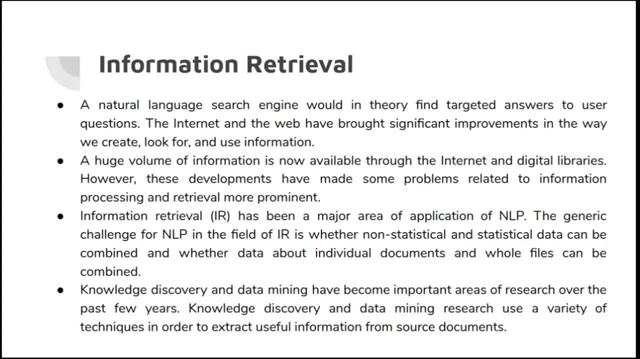 The internet and web have brought significant changes. A huge volume of data is available through the internet. However, this has made problems related to information processing. Information retrieval has been a major area in application of NLP. The challenge for NLP in field of information retrieval. 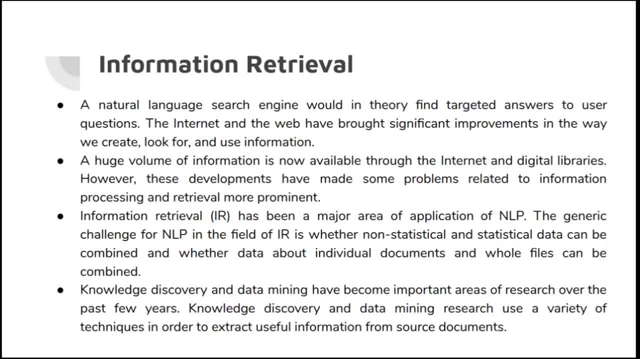 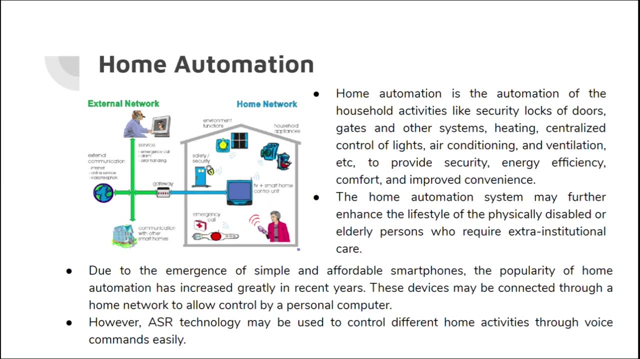 is whether non-statistical data and statistical data can be combined or not. Knowledge discovery and data mining research use a variety of techniques to extract useful information. Hello everyone, I'm Gaurav. Now let's discuss about the next application of automatic speech tracking. 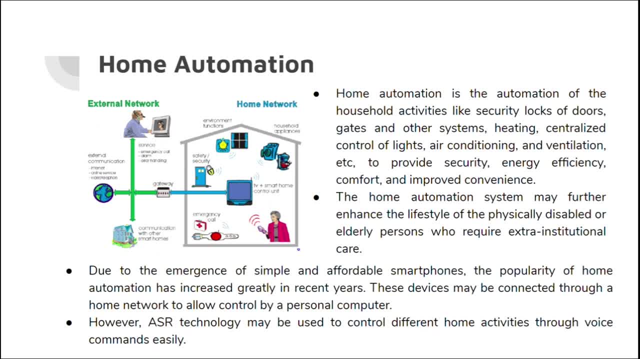 We are going to talk about Home Automation, which is Home Automation. So, first of all, what is Home Automation? Home Automation is basically the automation of all household activities, like security of doors or the working of your television, your air conditioning. 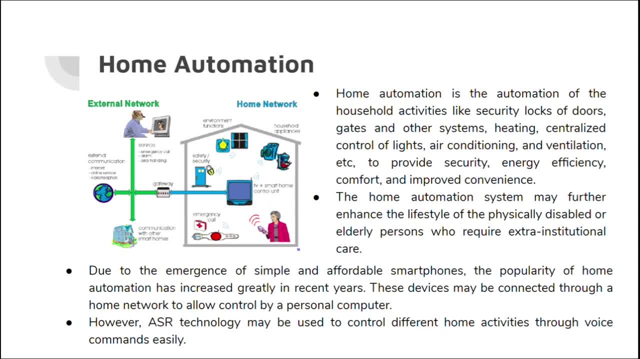 the lighting lights of the house, your fans, etc. everything. So, first of all, let's discuss what are the Home Automation tools that we use currently. So the Home Automation tool is called Home Automation. So the Home Automation tool is called Home Automation. 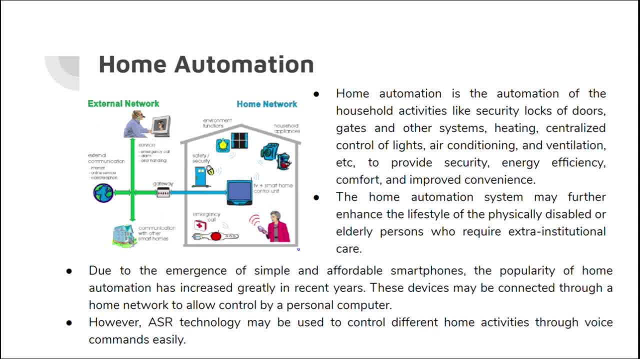 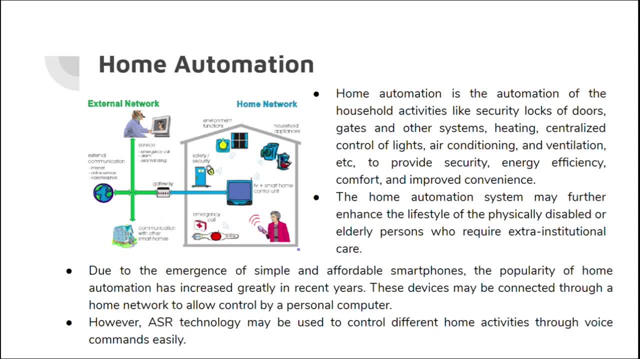 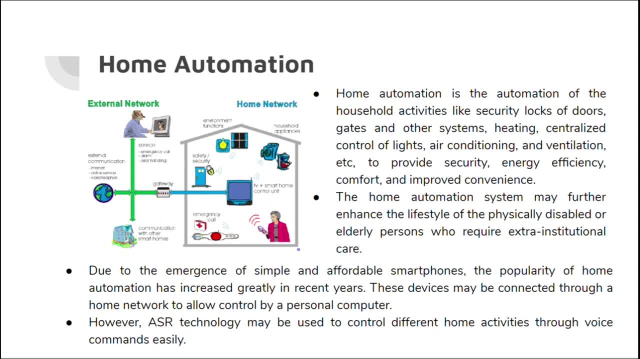 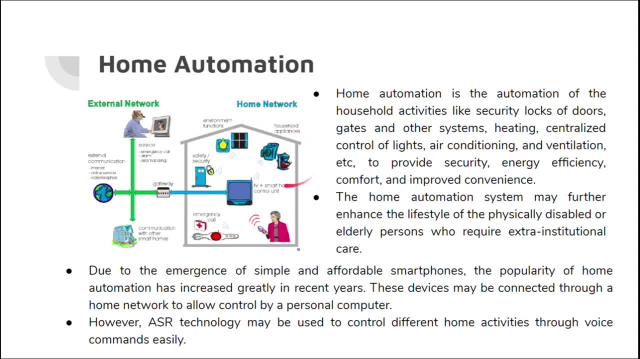 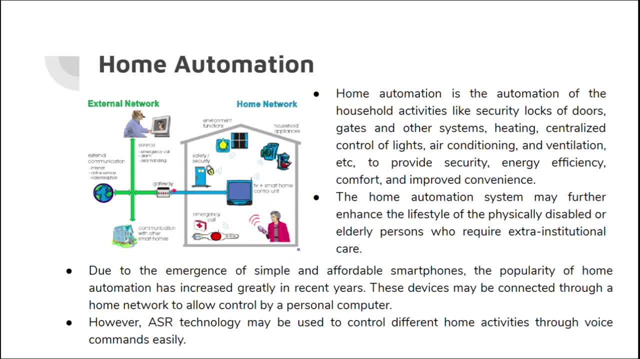 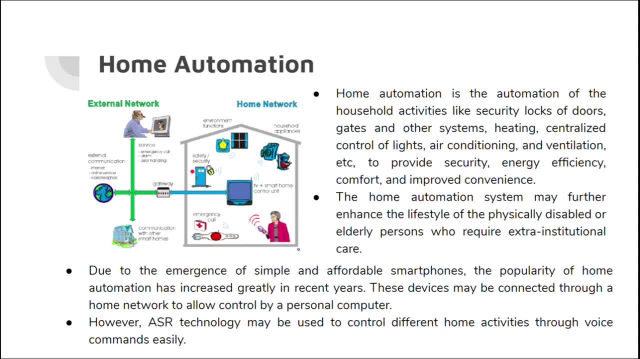 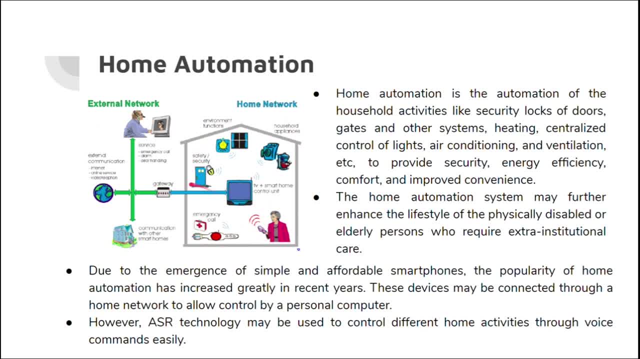 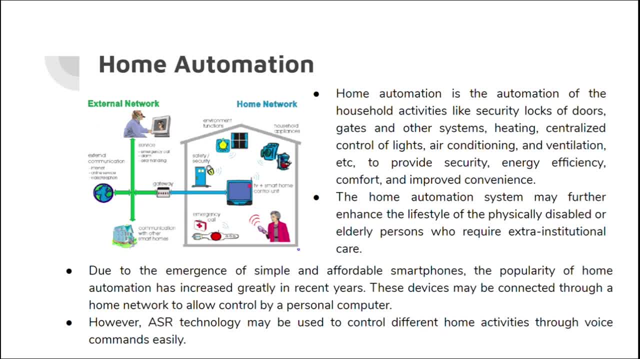 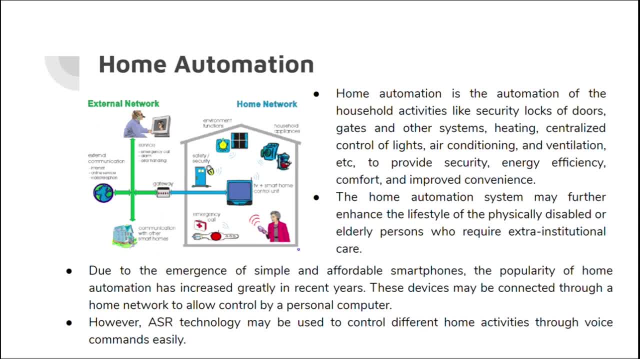 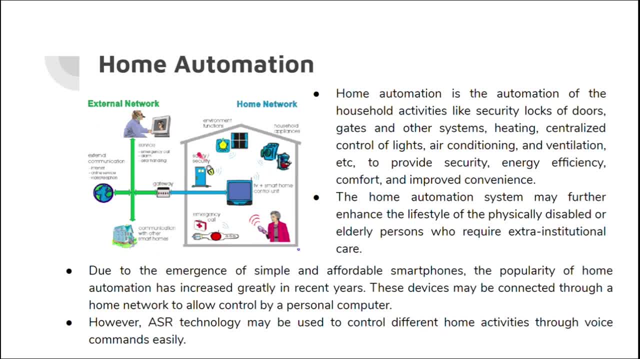 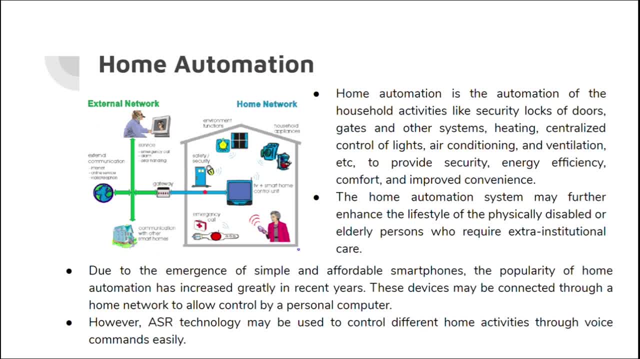 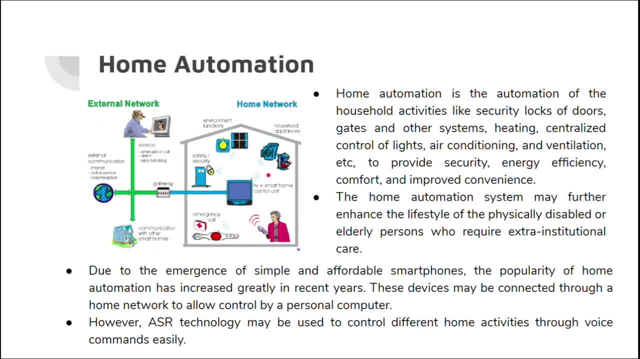 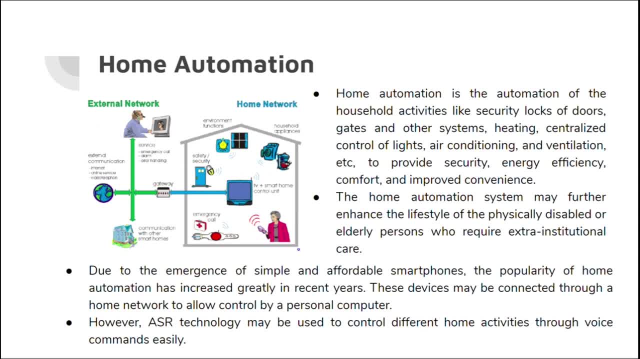 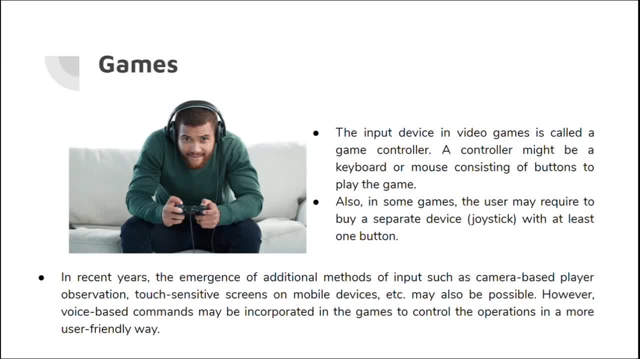 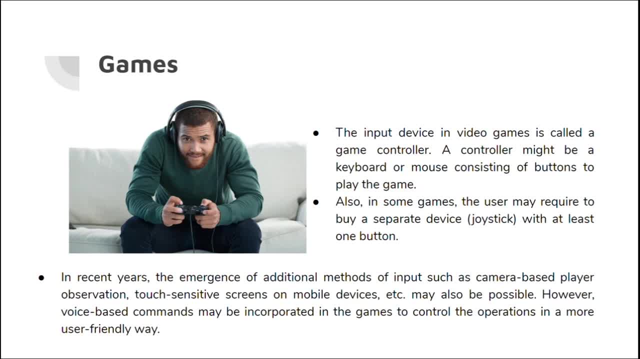 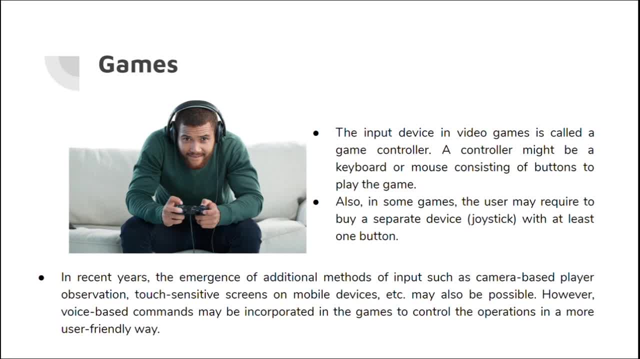 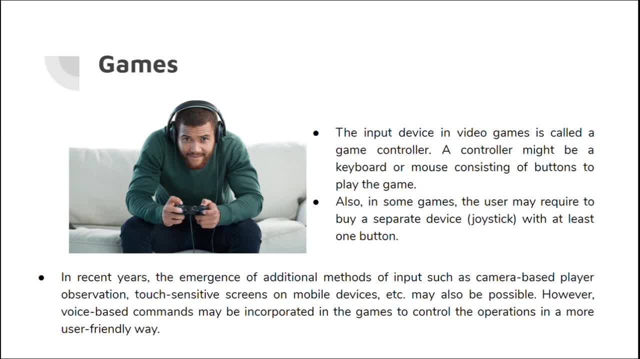 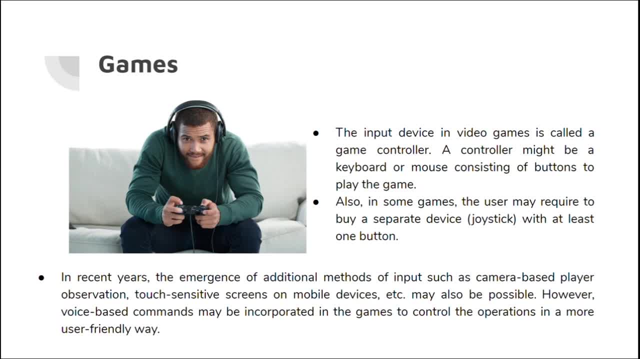 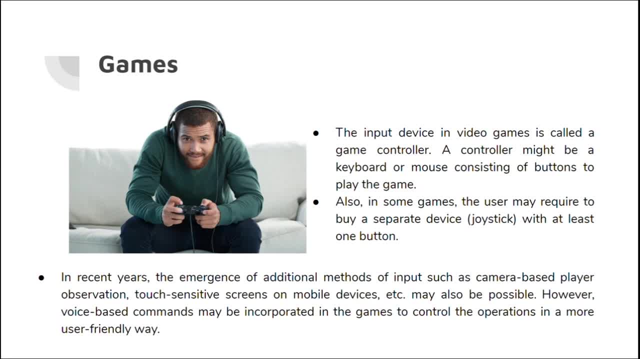 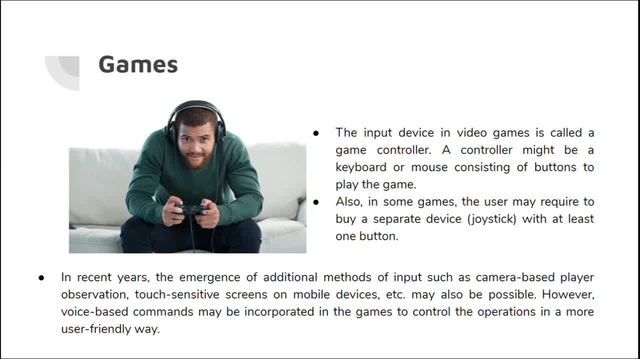 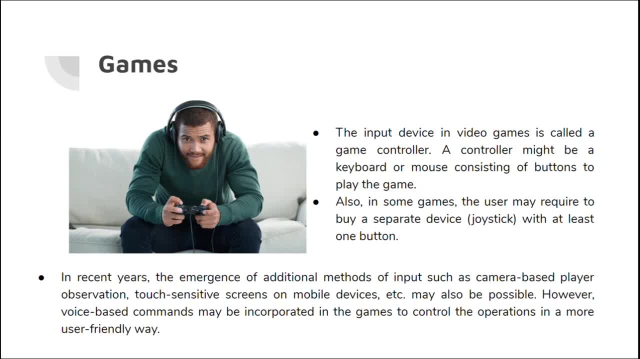 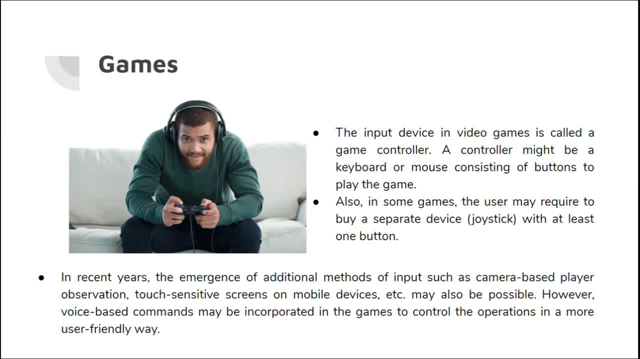 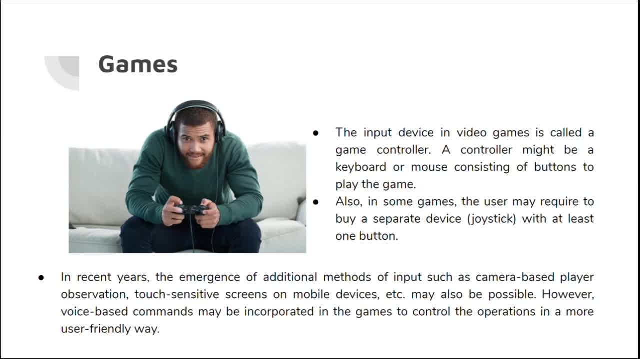 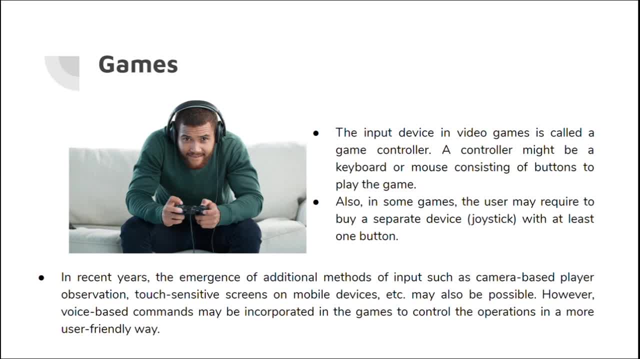 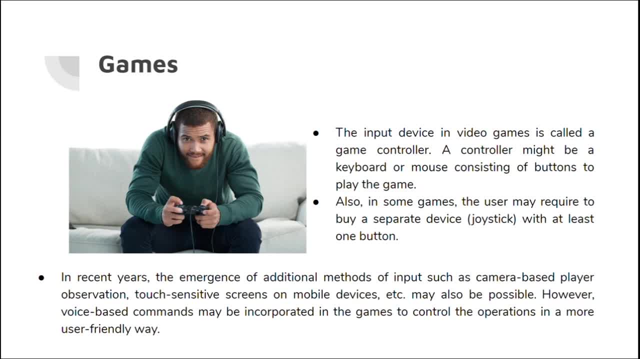 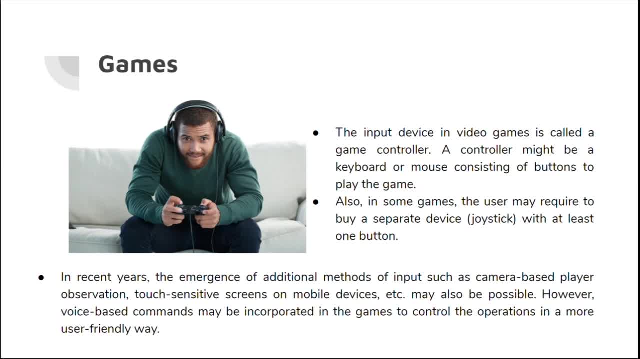 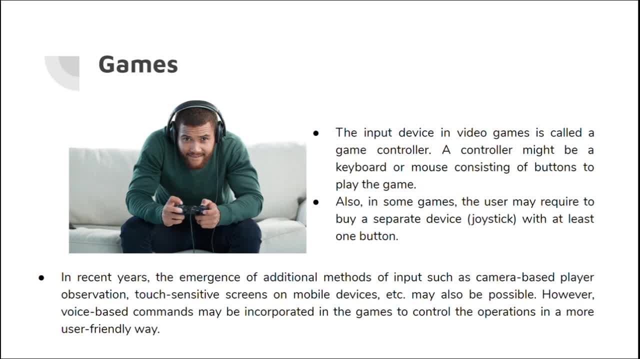 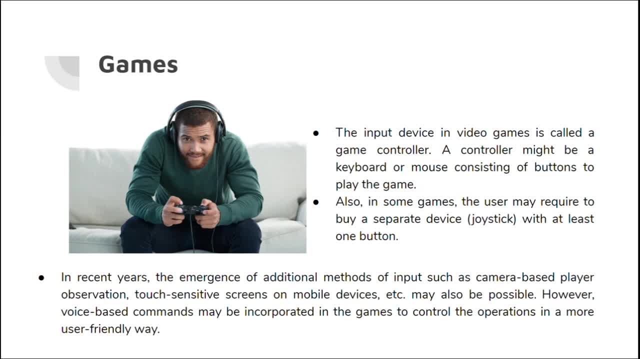 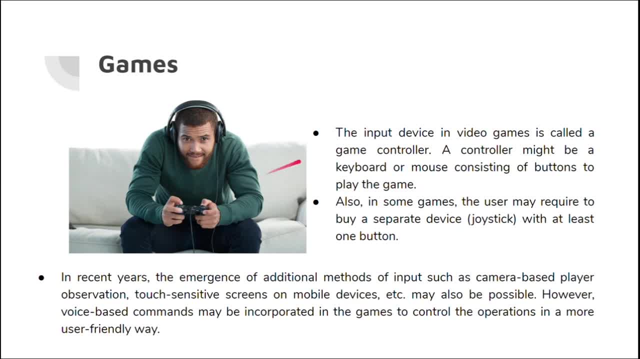 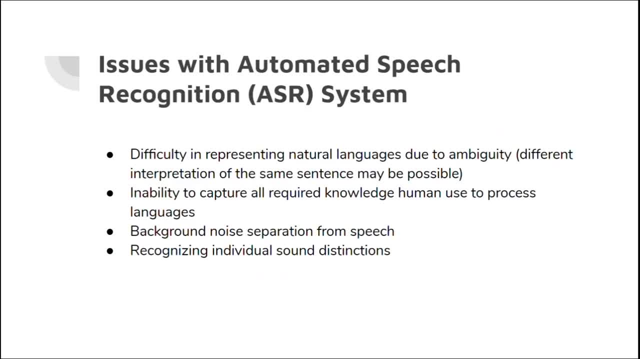 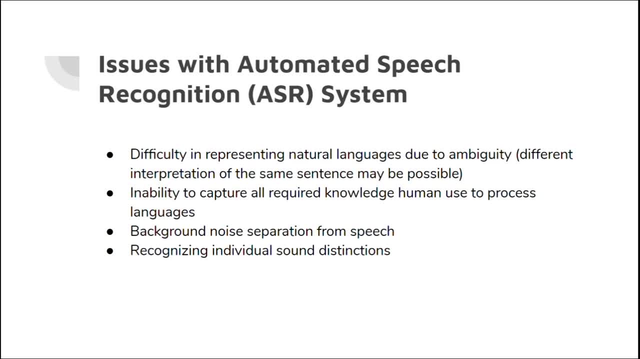 we have is difficulty in representing natural languages to the ambiguity. so humans tend to speak a lot using sarcasm, especially when they are communicating with some someone known to them. so in such cases it is very difficult for a machine to judge whether the person is saying something seriously or is it supposed to be sarcasm. next is inability to capture all required. 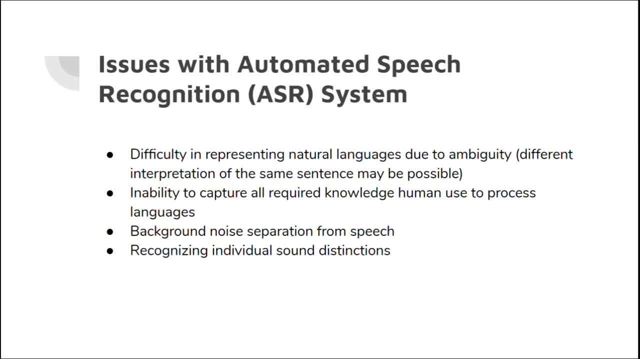 knowledge. human uses to process languages. this is about the fact that when humans talk, there is a lot of context that comes into play when they are communicating. however, it is practically not possible for a machine to have that entire context, so that that is why we say that it is enabled to. 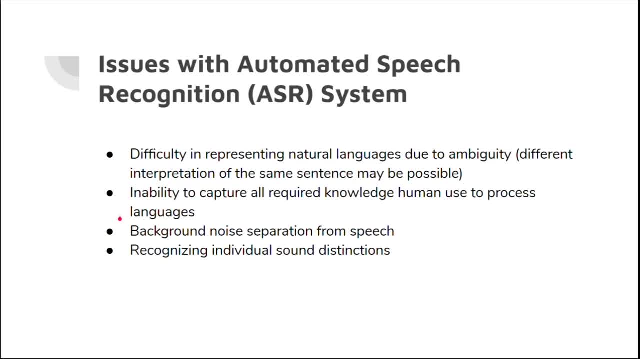 capture all of the required knowledge. next we have background noise, separation from speech. so this is basically like if you are in an outdoor situation where you are trying to give a voice command, there would be a lot of background noise and it is often very difficult for a machine to separate that voice.